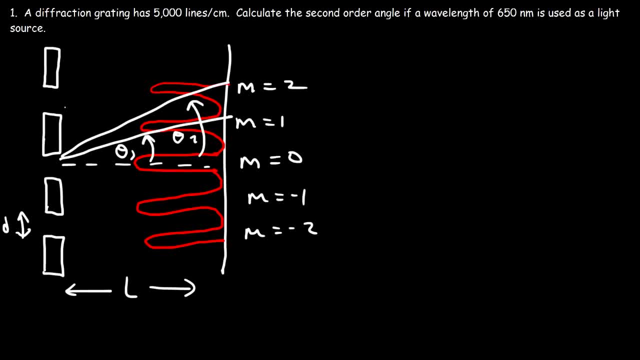 the diffraction gradient. now, the diffraction gradient has slits that are equally spaced and parallel to each other, and so a machine can be used to create all of these slits within a very small space. there's 5,000 slits per centimeter, so they're very close to each other. each slit is very, very small. 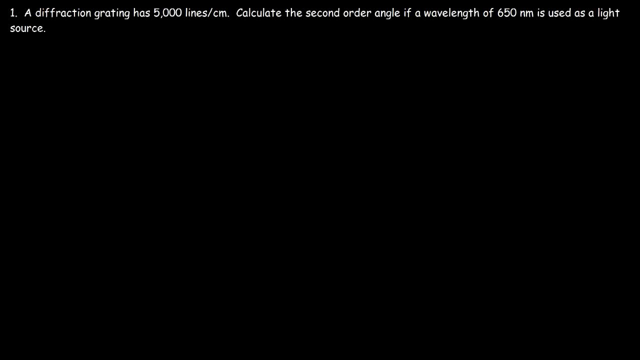 the main formula that we need to use is this equation: D sine theta is equal to M times lambda. now D is equal to 1 over n, where n represents the number of lines per meter. so let's calculate this thing first. so the diffraction gradient has: 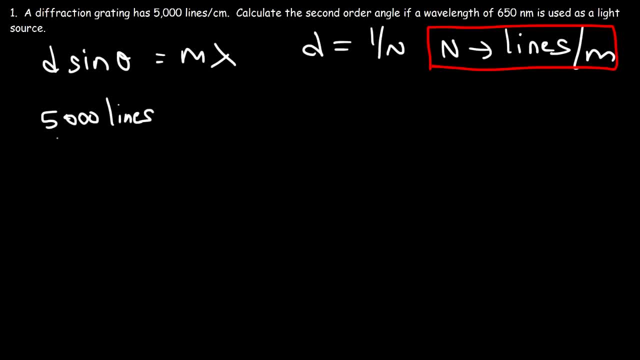 5,000 lines per centimeter. now let's convert centimeters to meters. there's 100 centimeters per meter, and so we could cancel these two, and so 5,000 times 100 is 500,000, which we could say it's 5 times 10 to the 5 lines per meter. so D is going to be 1 over n, so that's. 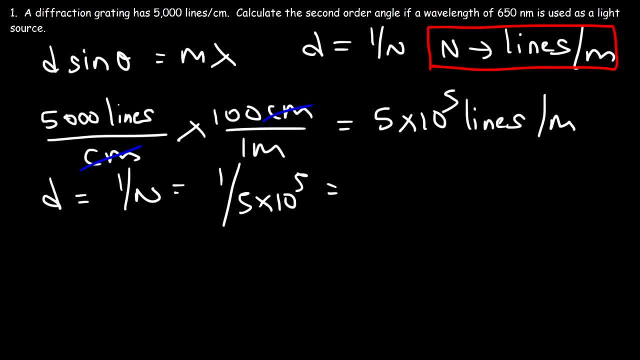 1 divided by 5 times 10 to the 5, and so this is equal to 2 times 10 to the minus 6 meters per line. so that's the spacing of each slit in this problem. so now that we have D, we can calculate. 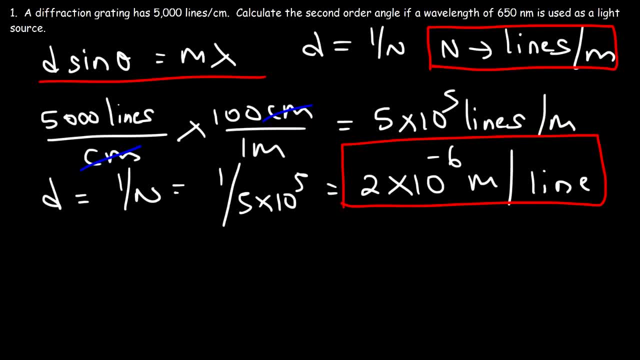 everything else. so let's make a list of what we know. so the second order angle, theta 2, is what we're looking for. lambda is 650 nanometers and, because we're dealing with a second-order angle, M is 2, so let's plug in everything into this equation. so d is 2 times 10 to the. 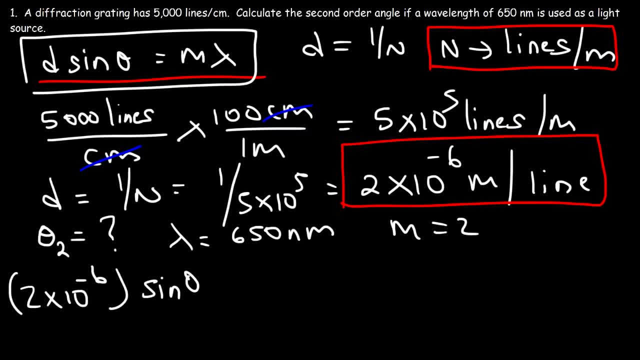 minus 6 times. sine of theta 2 M is 2 and lambda 650 times 10 to the minus 9. so let's take 2 and multiply it by 650 times 10 to the negative 9, and then divide that by 2 times 10 to the minus 6.. So we get that sine of theta 2 is 0.65.. So theta 2 is going. 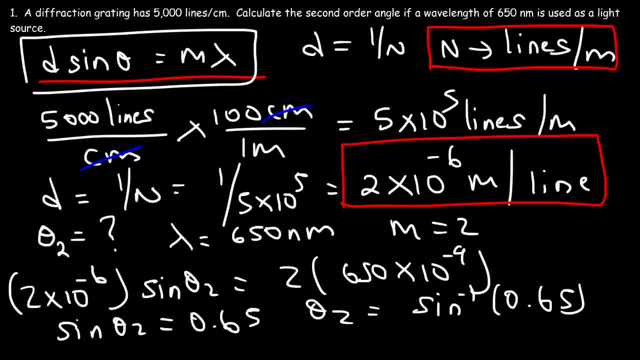 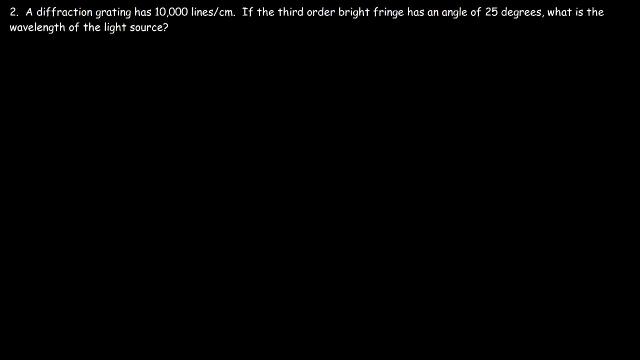 to be arc sine of 0.65, or the inverse sine function, And so the answer is 40.5 degrees. So that's the second order angle for this diffraction gradient if we use a wavelength of 650 nanometers. Number two: a diffraction gradient has 10,000 lines per centimeter. 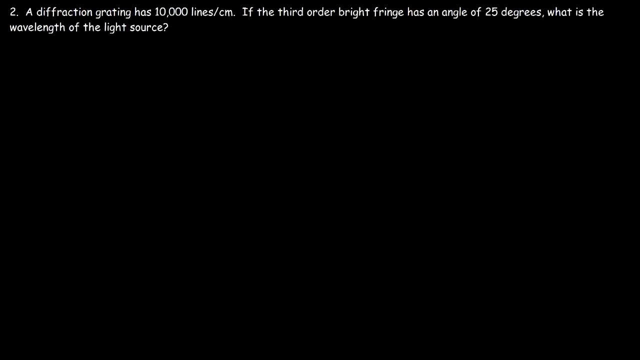 If the third order, bright fringe, has an angle of 25 degrees, what is the wavelength of the light source? So, based on the last example, feel free to pause the video and work on this one. So let's start with: okay, let's redo that. 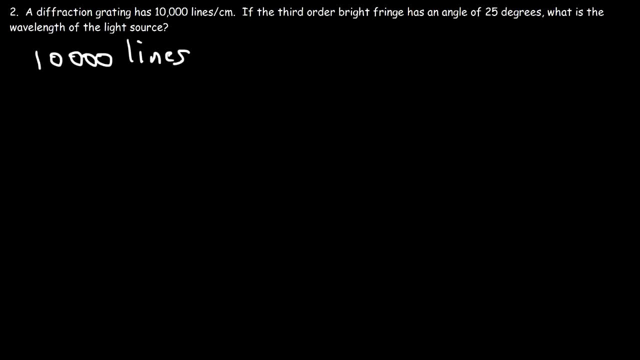 Let's start with 10,000 lines per centimeter And let's convert centimeters to meters, just like we did before. So one meter is equal to 100 centimeters, And so 10,000 times 100 is a million. 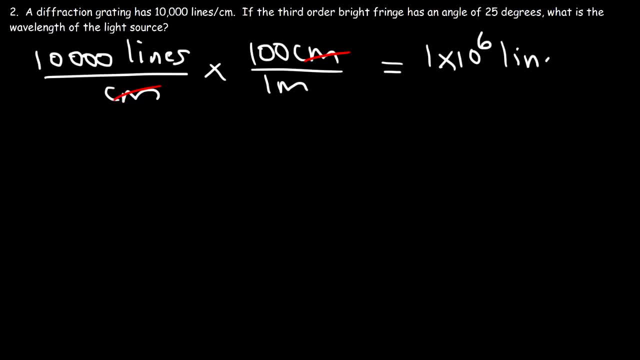 which is the same as one times 10 to the six lines per meter. Now D is equal to one over N And this quantity is equal to N, So D is gonna be one divided by one times 10 to the six, which is one times 10 to the negative six. 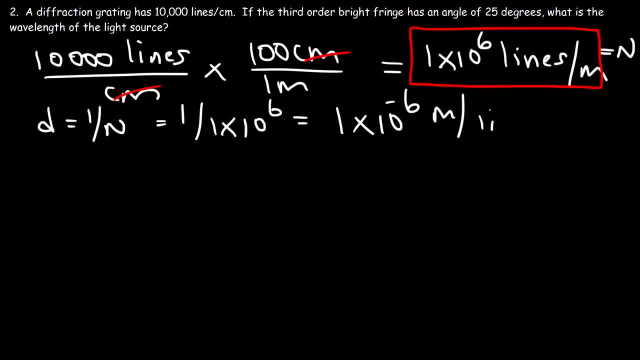 And we're gonna flip the units, so it's gonna be meters per line. So that's the spacing of each slit. So now let's make a list of what else we know. So the third order angle is 25 degrees, And so M has to be three. 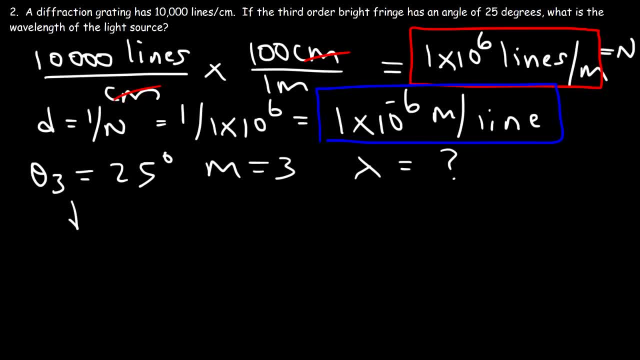 Our goal is to calculate the wavelength, So let's use the formula D sine theta is equal to M times lambda, So D is one times 10 to the minus six, And then it's gonna be times sine of 25 degrees, And then it's gonna be times sine of 25 degrees. 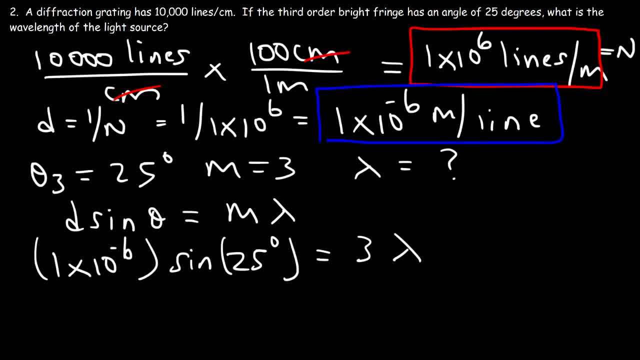 That's equal to three times lambda. So let's multiply one times 10 to the minus six by sine 25, and then divide that result by three. So the wavelength is 1.41 times 10 to the negative seven meters. Now let's convert this to nanometers. 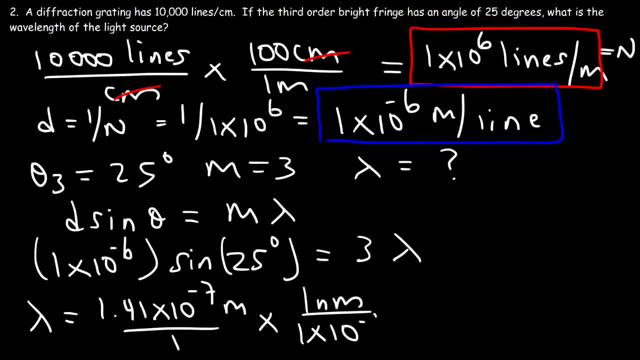 So one nanometer is one times 10 to the negative nine meters. So we need to take 1.41 times 10 to the minus seven and divide it by 10 to the negative nine, And so the wavelength is 141 nanometers. 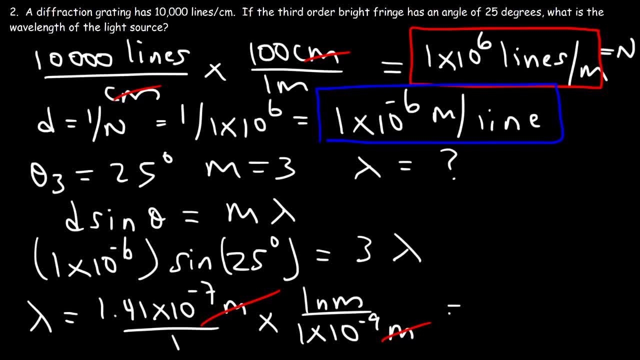 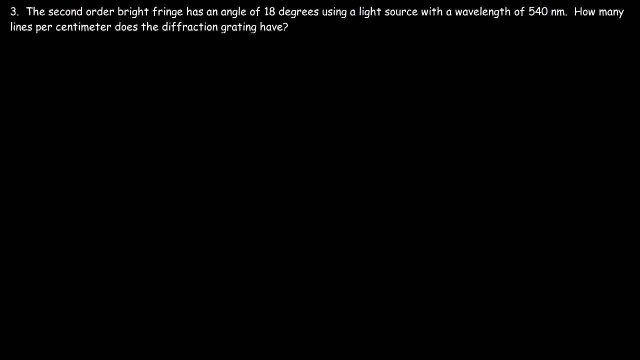 So this is the answer to the problem Number three, the second order bright fringe has an angle of 18 degrees using a light source with a wavelength of 540 nanometers. So the second order of bright fringe has an angle of 18 degrees using a light source. 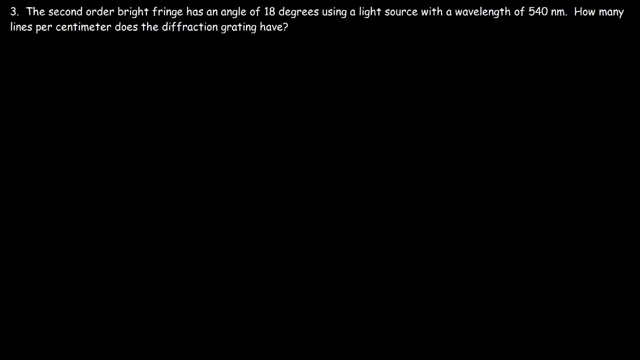 with a wavelength of 540 nanometers. So this is the answer: How many lines per centimeter does the diffraction gradient have? So what do you think we need to do in this problem? Go ahead and work on it. So let's make a list of what we know. 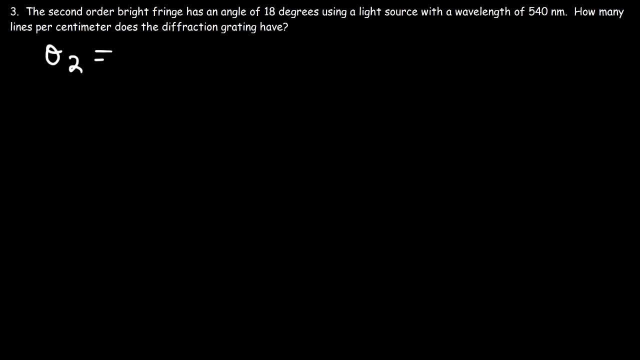 So the second order bright fringe, or the second order angle is 18 degrees. The wavelength is 540 nanometers. Now, because the subscript is 2, we know that m is equal to 2. So if we can calculate d, we can then calculate the number of lines per centimeter. 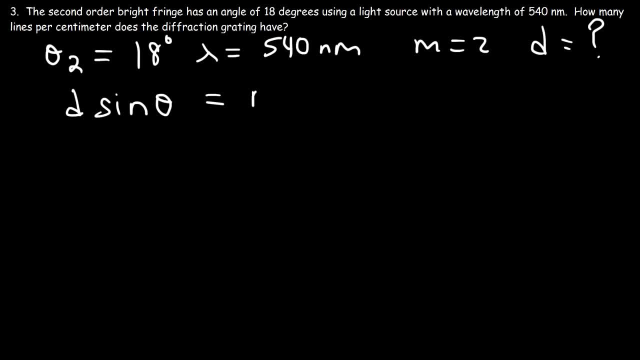 So let's use this equation d sine: theta is equal to m times lambda. So theta is 18 degrees, m is 2, and lambda is 540 times 10 to the negative 9.. So let's multiply those two numbers. 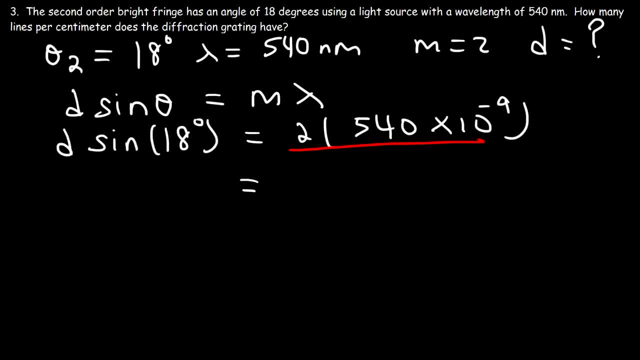 And so that's going to be 1.08 times 10 to the negative 6.. Now let's divide both sides by sine of 18 degrees, And so now we have d, which is 3.4.. So that's going to be 1.08 times 10 to the negative 6..